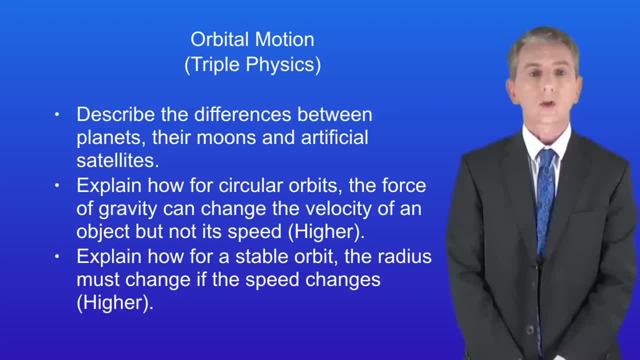 the velocity of an object, but not its speed. Higher tier students should also be able to explain how, for a stable orbit, the radius must change if the speed changes. and all of this is for triple physics students only. Okay, I'm showing here the earth orbiting the sun. Scientists call this a. 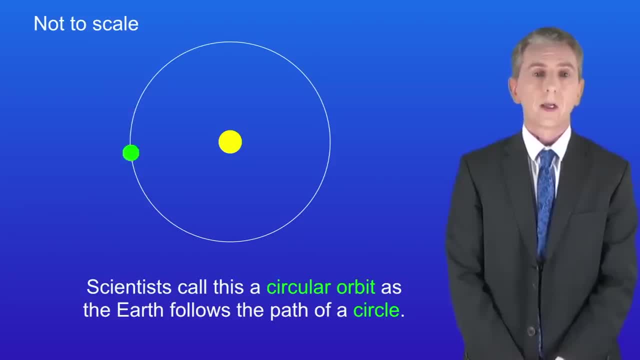 circular orbit, as the earth follows a path of a circle. Now, strictly speaking, planets actually orbit the sun more like this. Scientists call this an elliptical orbit. However, in this video, we're only looking at circular orbits, and I should point out that the earth's orbit is virtually circular. 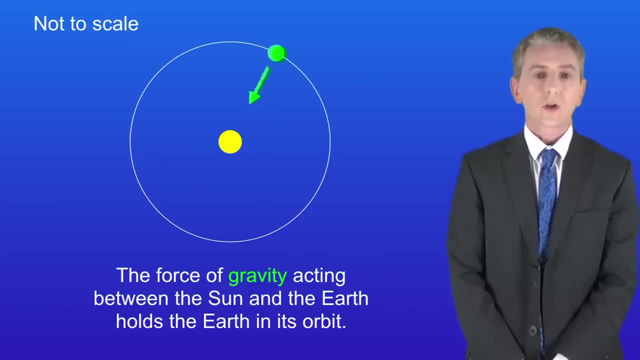 The force of gravity acting between the sun and the earth holds the earth in its orbit and the arrow shows a force of gravity. So the key point is that planets orbit the sun and the force of gravity holds the planets in their orbits. Okay, I'm showing you here the moon in a circular orbit. 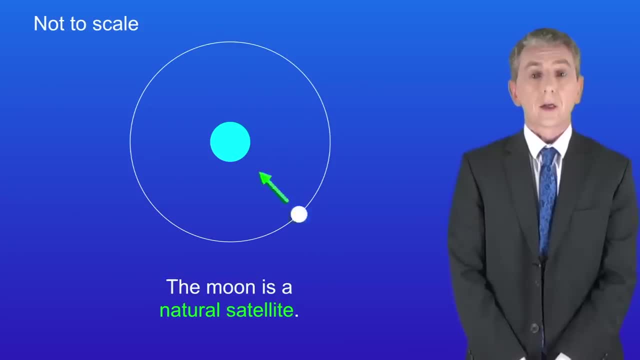 around the earth. Now the moon is a natural satellite. Once again, the force of gravity holds the moon in its orbit. Okay, this shows an artificial satellite, For example, the type used for satellite tv. Artificial satellites are man-made Geostationary satellites orbit once every 24 hours. This means 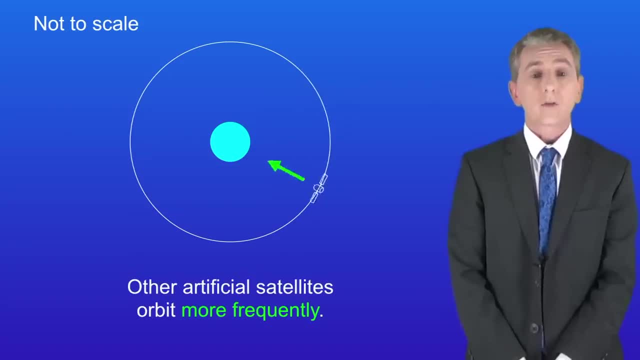 that they always point to the same part of the earth. However, other artificial satellites orbit more frequently. Now, as we said before, the force of gravity holds objects in their orbit. A key point is that in the case of circular orbits, the force of gravity is leading to a change in velocity. 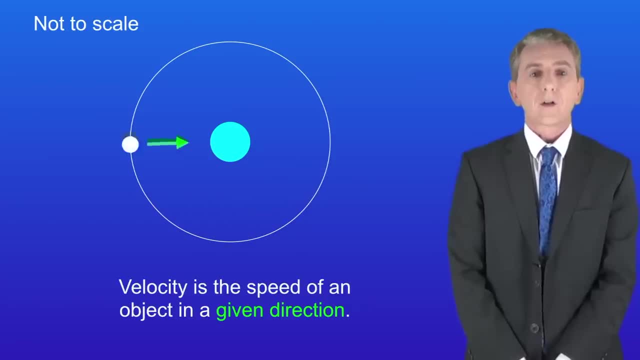 but not a change in speed. Remember that velocity is the speed of an object in a given direction. This red arrow shows the direction that the objects move in. As you can see, the direction is constantly changing, So this means that the velocity is constantly changing as well. However, 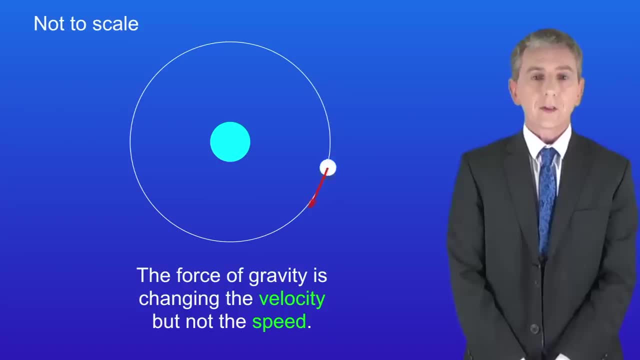 you'll notice that the speed is constant. So the force of gravity is changing the velocity, but not the speed. Okay, we're going to look now. one final point. I'm showing you here a satellite orbiting the earth. If the speed of the satellite changes, then the radius of the orbit must also change. 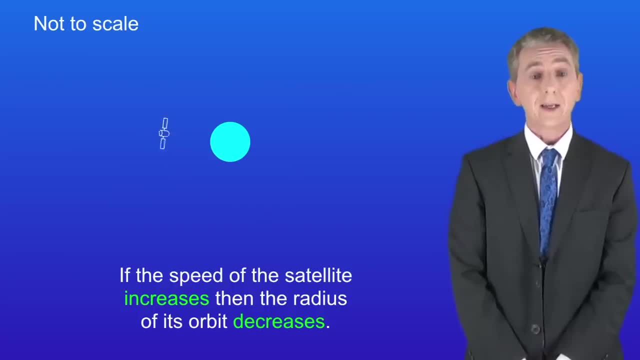 So if the speed of the satellite increases, then the radius of its orbit decreases. That's because at a higher speed the satellite needs a greater force of gravity to prevent it flying off into space. So by moving closer to the earth the gravitational force on the satellite is greater.